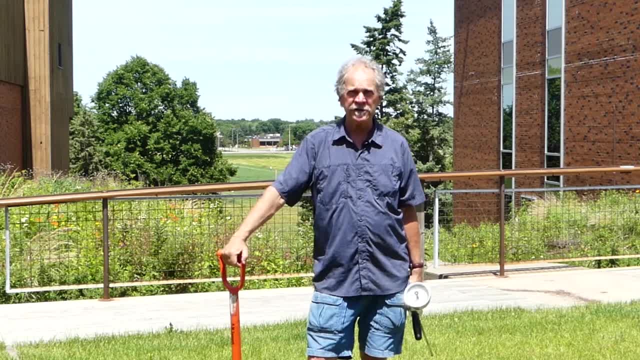 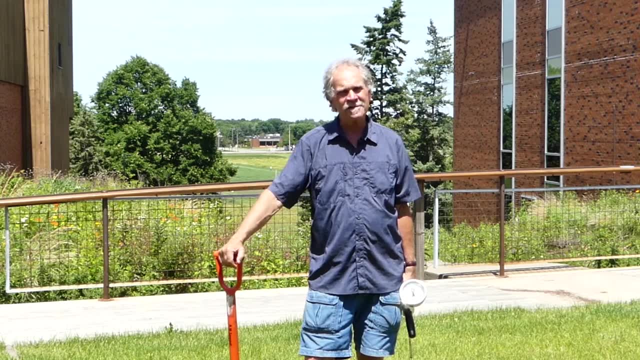 a couple different ways we can measure. If you remember one of the other segments, or go forward to one of the other segments, when we tested for percolation of water in the soil, we actually weren't testing for water, We were testing for oxygen. What is the ease? 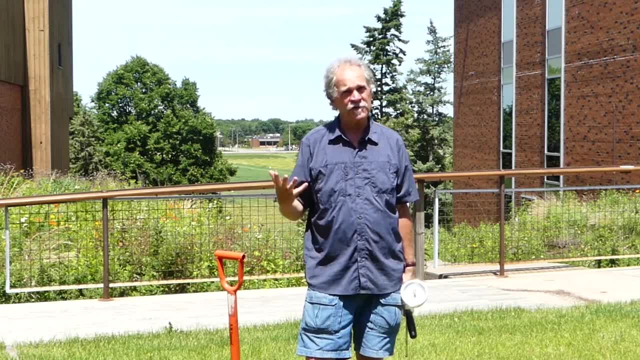 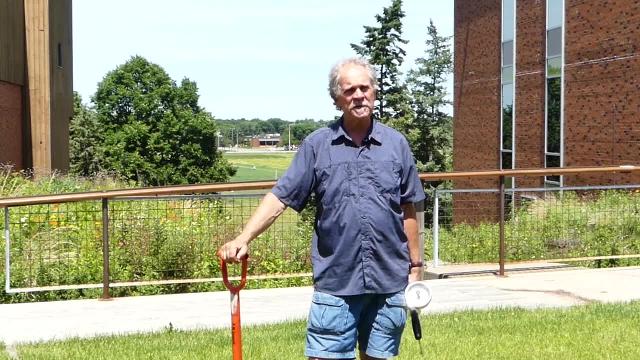 for the oxygen to diffuse through the soil, And if the soil is waterlogged, it's very difficult for oxygen to diffuse through the soil. One of the things that has been found in many, many, many years of research is that there are a lot of studies that show that. 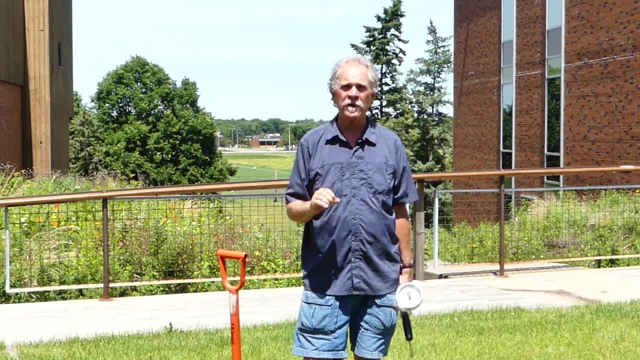 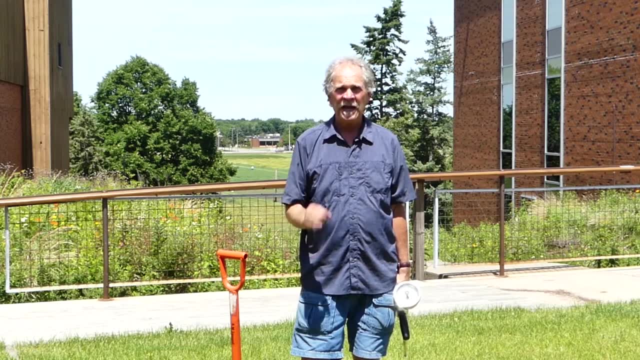 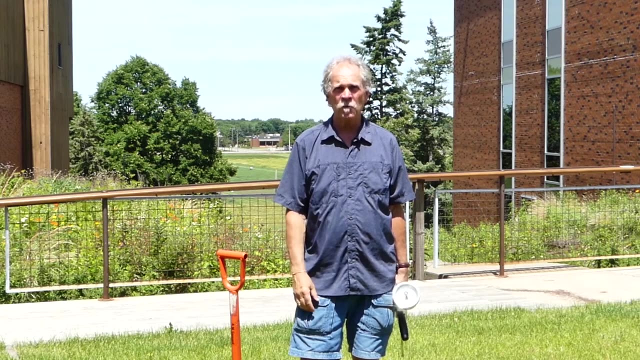 this is the case. Kind of the definitive test for whether or not a tree is going to survive and be healthy is what's called the oxygen diffusion rate, And that oxygen diffusion rate is a function of a couple things. One, is the soil waterlogged? If it's waterlogged, 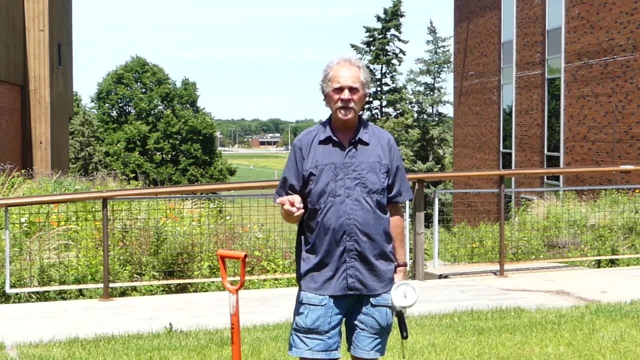 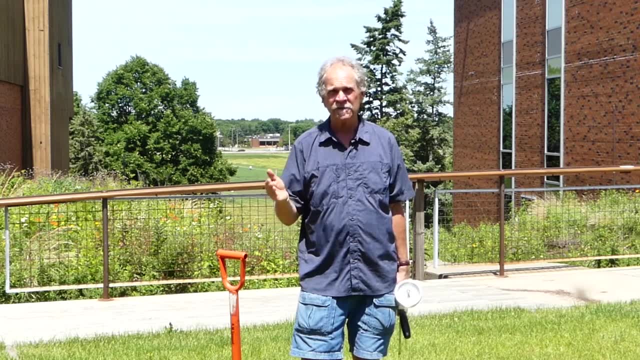 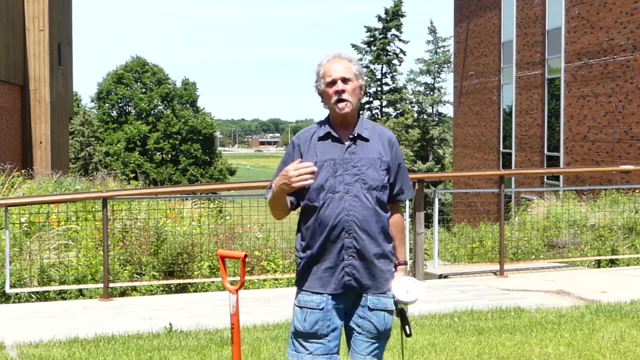 oxygen can't diffuse normally. And then, second of all, is the soil compacted? specifically, if it's compacted and it's a clay soil, Same problem. It's very difficult for oxygen to diffuse horizontally in the soil. So there are a couple of ways we can test for it before. 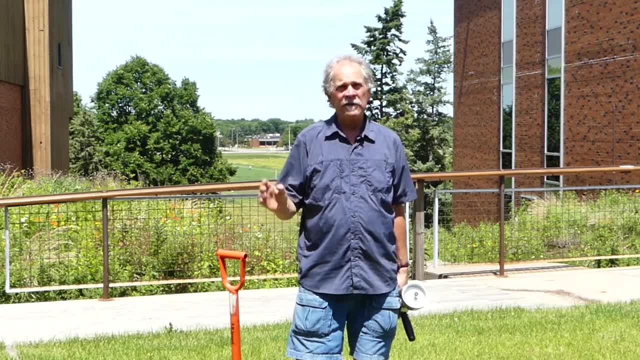 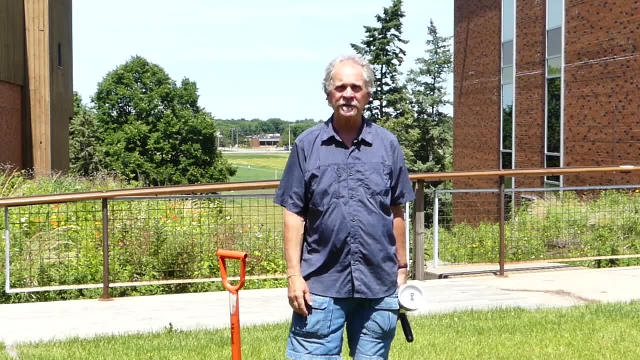 we select the trees that we're going to plant here, Or if we are just determined to have a tree like a sugar maple that doesn't do well in compacted soil, what we're going to have to do to the site to make sure we increase that oxygen diffusion rate, One of the instruments 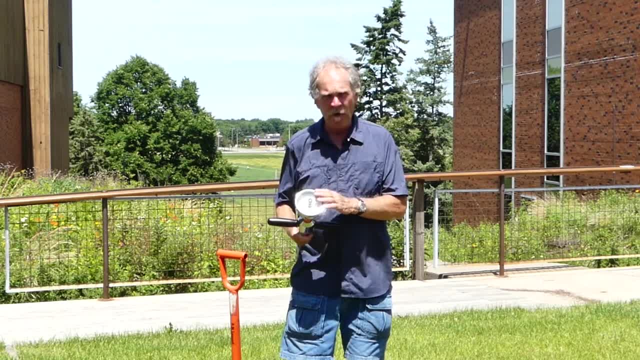 we use is a penetrometer, And from research we know that once you get over 400 foot-pounds of resistance, you're going to have a lot more oxygen to diffuse in the soil, So we're going to have to increase that oxygen diffusion rate. One of the instruments we use is a penetrometer. And from research we know that once you get over 400 foot-pounds of resistance, you're going to have a lot more oxygen to diffuse in the soil. So we're going to have a lot more oxygen to diffuse in the soil. So we're going to have a lot more oxygen memoir, And that's what I'm going. 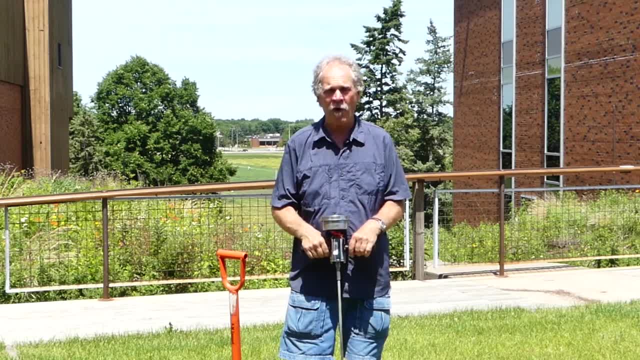 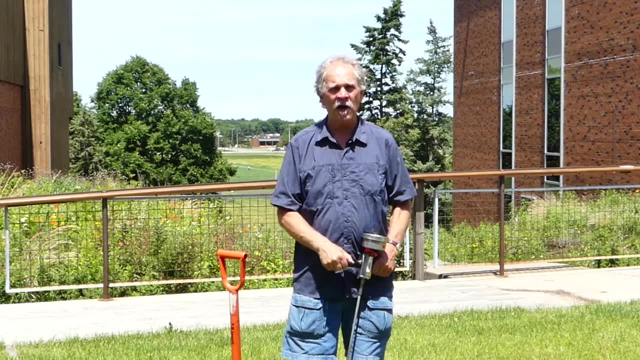 to be doing is testing resistance as I push this into the ground. Once you hit over 400, it starts slowing roots down, Makes it a little bit more difficult for them to expand out. If it's more difficult for them to expand out, they don't grow as fast, they don't take up as much water. They're. 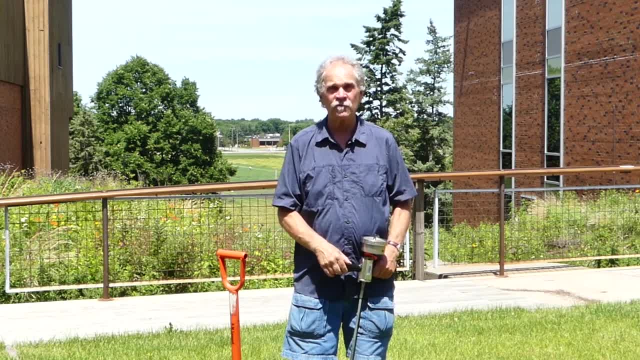 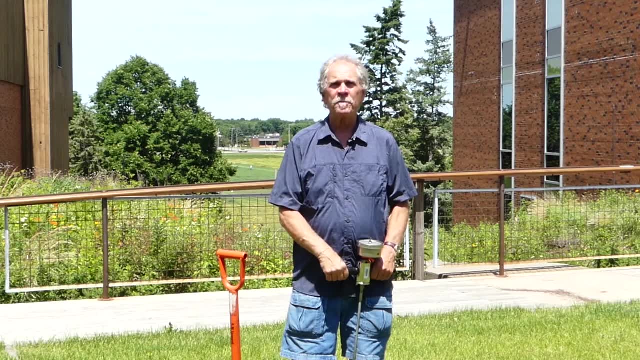 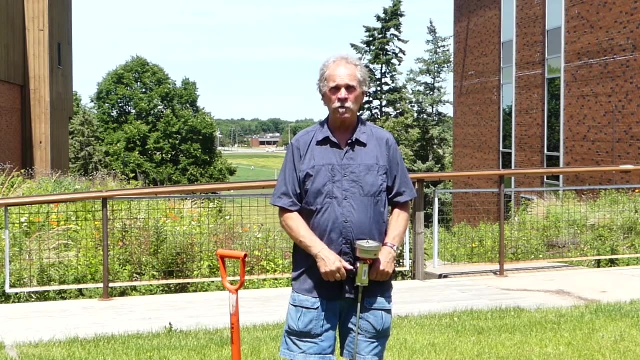 a little bit more vulnerable to changes in the climate or a dry season. We have had some of our test sites in a metropolitan area and public parks where the penetrometer reading has been 1,300, greater than 1,300, which is really difficult for roots to penetrate.